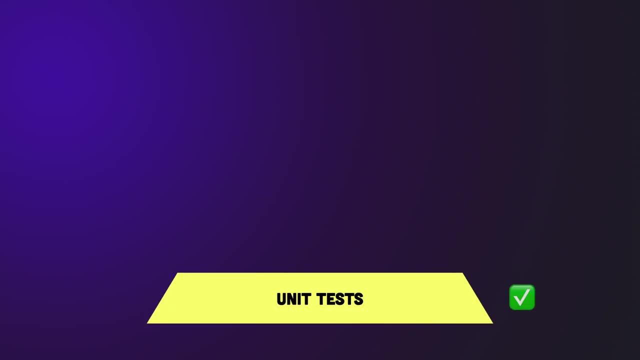 You would assume that if everything is working at the lowest level, then it's all going to work when you put it together. but that isn't always the case, which is why we need the next level of tests. The next level up in our testing pyramid is what we call component tests. This is where we test. 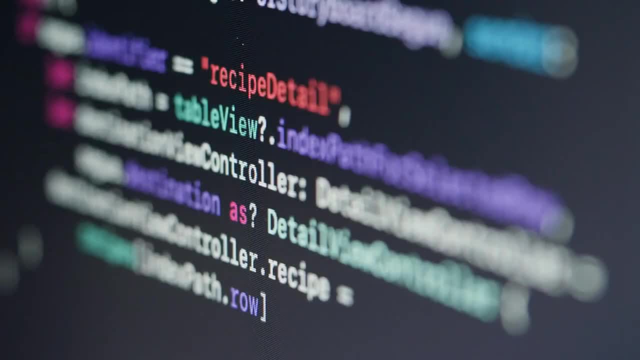 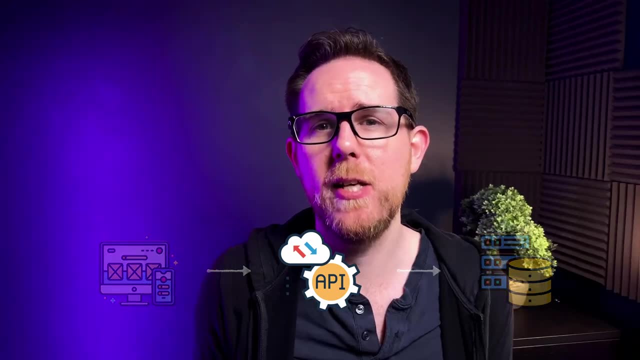 a complete section of your application. For example, if you're writing a web application, you might have a front end, an API and a database. A component test for the API would therefore test the API in isolation from all the other components. We wouldn't include the front end, for example, and 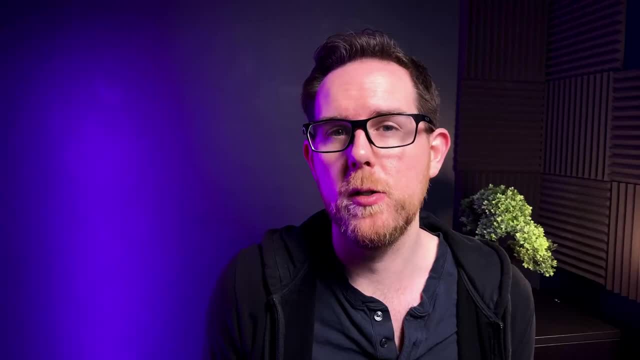 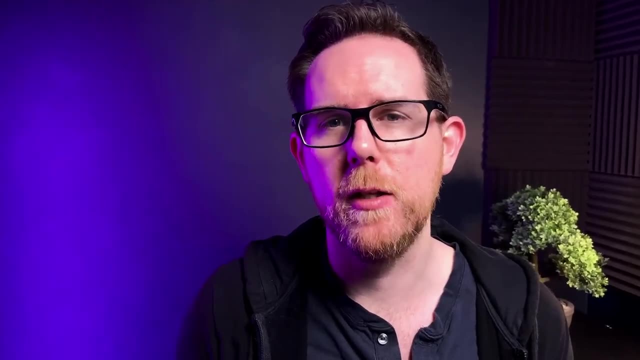 we'd also mock out the database, as well as any other components that you'd want to test. The purpose of the component test is to make sure that your application is doing what you expect it to do, without the interference of the other components. By mocking out the 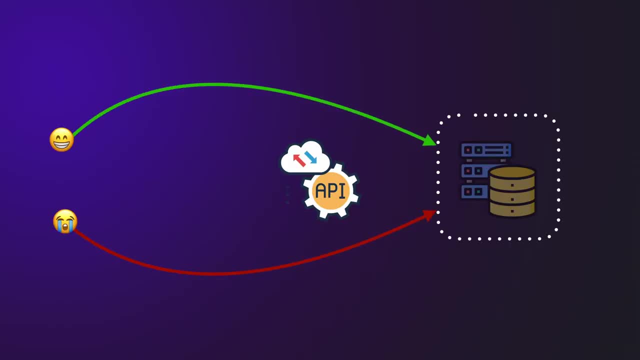 database. we can test both the happy path and the unhappy path of your application. We can see how the application will behave under certain conditions, such as if the database is down or if you send in a bad request. Component tests make sure that all those units that 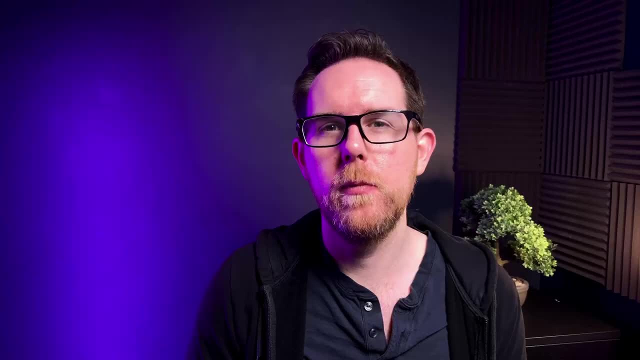 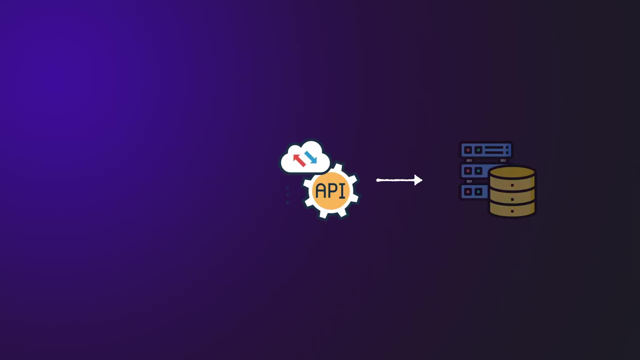 you tested in the previous level work well when you put them together. The next level on our testing pyramid is what we call the integration tests. In the previous level we mocked out the database and other factors, but here we want to make sure that those integrations actually work. This is where you'll usually find out that the team that 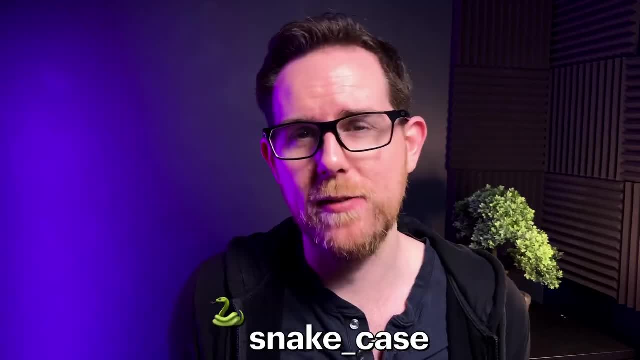 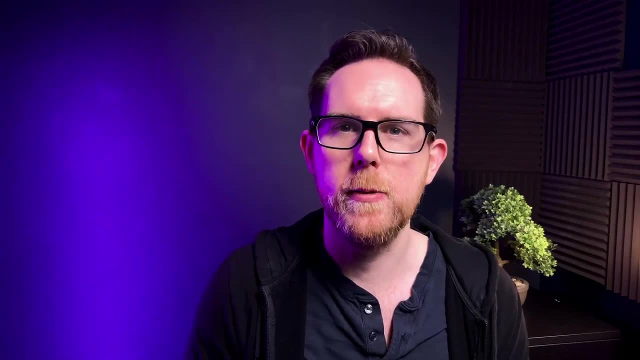 you've been working with have decided to use camel case instead of snake case for their API. The monsters: Or you'll find out that you have the connection string wrong for your database, or you've written a typo in one of your SQL queries. For all these tests that we've done, so far. we generally don't do them on an actual environment. Unit tests, component tests and integration tests are all generally run as part of the build process or at the very least, before a release. Thanks to docker, it's fairly easy to spin up a database and use it when you're running. 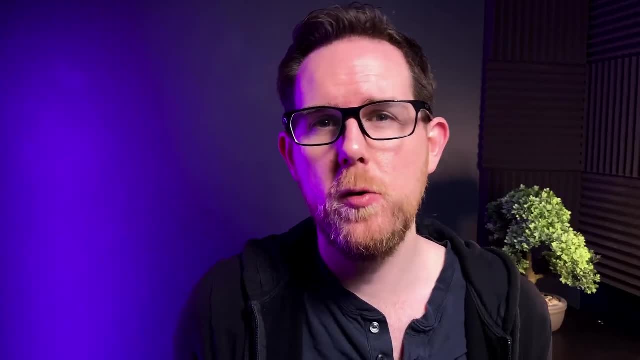 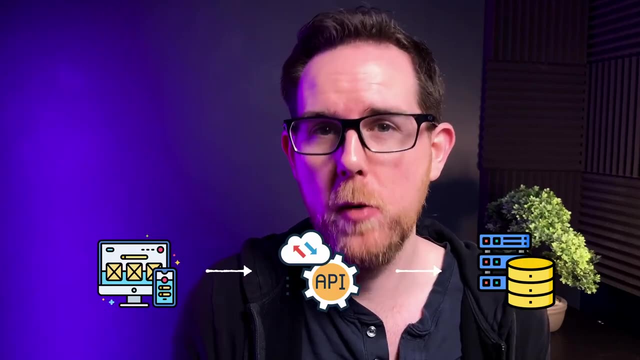 your tests on your CICD server. A lot of developers get confused by integration tests, thinking they need to test all of their application, but that isn't the case. You just need to test the integrations between your components. Generally, depending on who writes your integration tests, 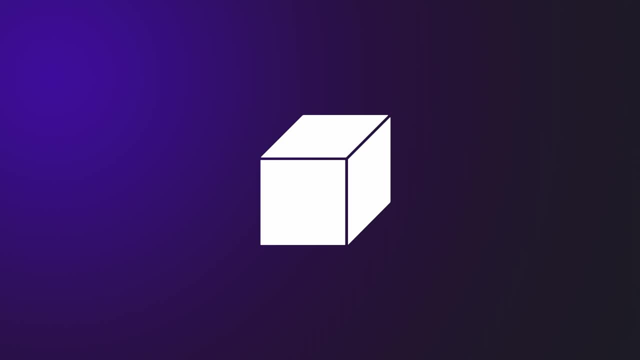 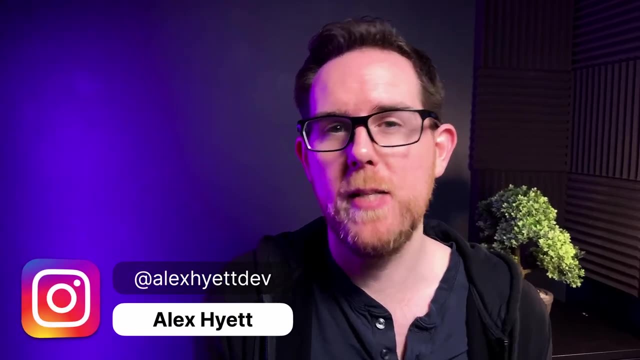 whether it be a developer or a tester will determine whether they're considered white box testing or black box testing. For example, if your integration tests are written by a developer and you're testing whether your database repository can correct your integration tests, then you can correctly write to your database. then this would be considered a white box test. However, if your 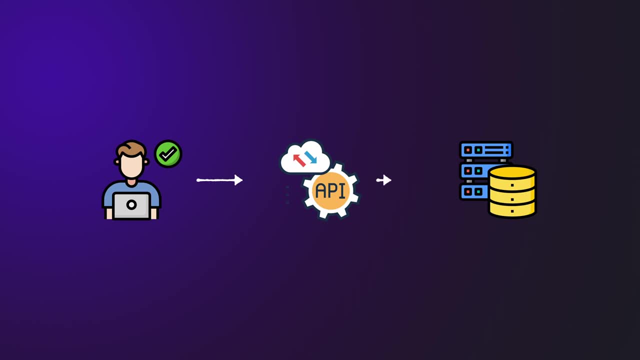 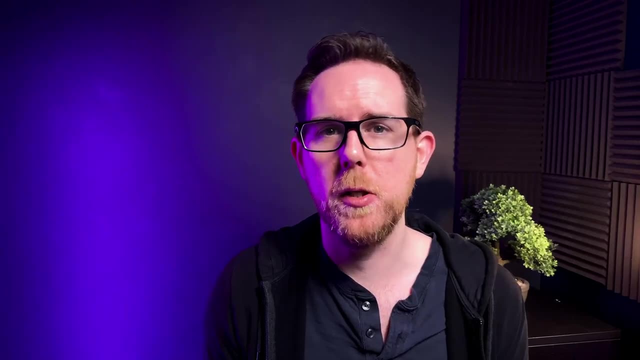 integration tests are written by a tester, then they might be calling the API and then seeing whether there's something in the database. This would therefore be more of a black box, because they don't need to know the internals of the application. It's not just the calls to the. 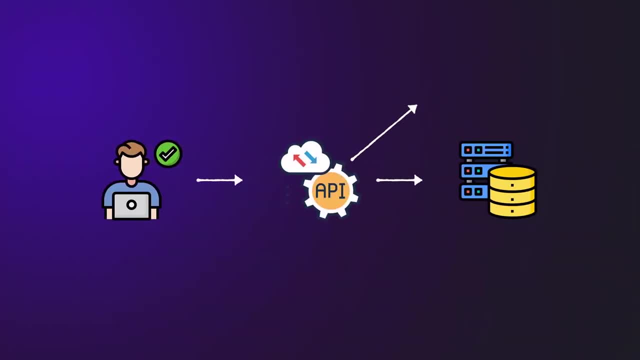 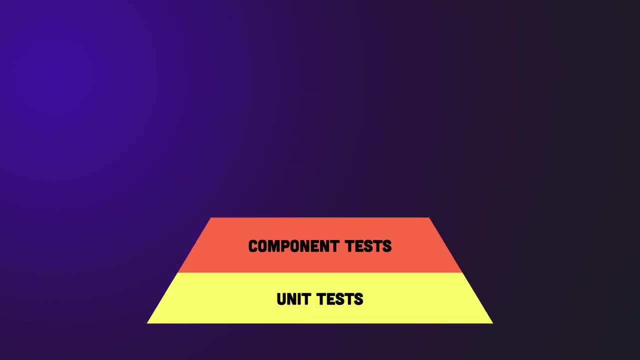 database that you might want to include in your integration tests. You also want to test things like calling other APIs, as well as writing a message to a message queue. So far, we've tested the individual functions, we've tested the components and we've tested how they interact. 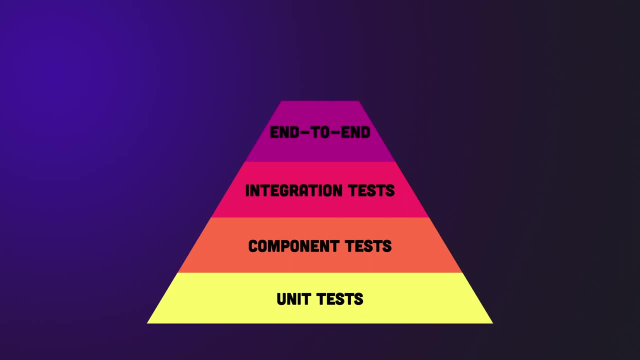 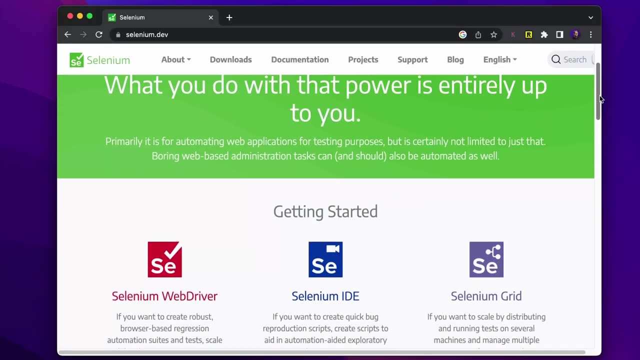 together. The next level is the integration test. The integration test is where you test the application from end to end. If you're writing a web application, then these will typically be in the form of automated UI tests, and we generally use tools such as Selenium or Cyprus to drive. 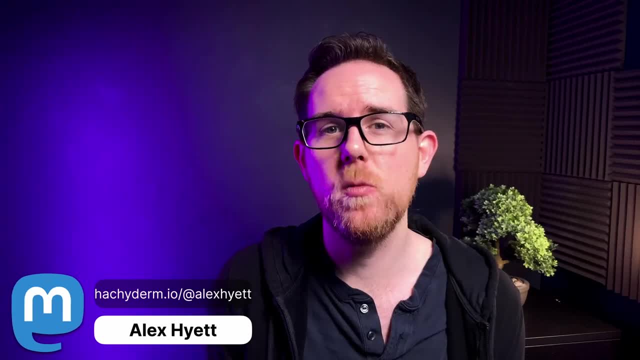 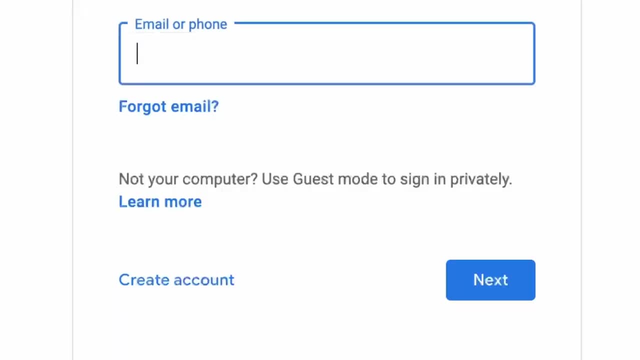 the UI through a web browser. The goal here is to test that everything is working as expected. End-to-end tests typically include a mix between functional testing, such as making sure the login works or a list is populated correctly, and acceptance testing, which makes sure that your 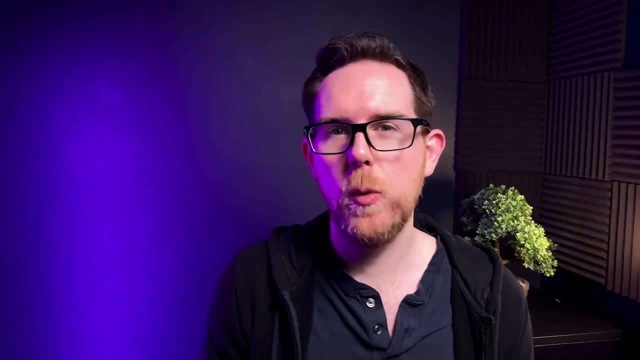 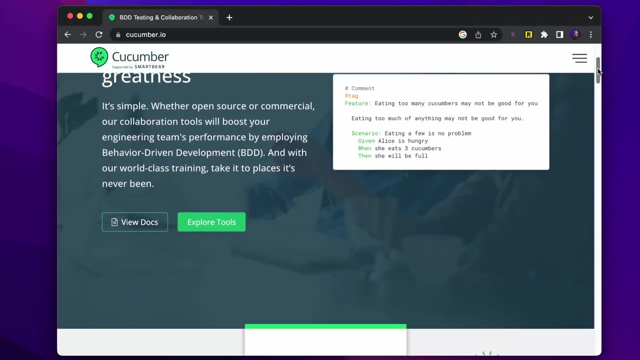 application is meeting business requirements, We tend to write end-to-end tests in what we call Gherkin language, which follows the given. when, then, pattern Frameworks such as SpecFlow and Cucumber allow us to execute code in this format while still having the tests understandable by, the business stakeholders. End-to-end tests can take a really long time to run and typically they're not run on every single build. Once you have a lot of them, they can take several hours to run, so you generally need to run them overnight. This isn't ideal if you want to be releasing. multiple times per day and therefore most teams split up their tests into multiple groups, with a critical group that they can run. If you want to run multiple times per day, then you need to run before each deployment, Unlike the other tests that we've looked at so far. 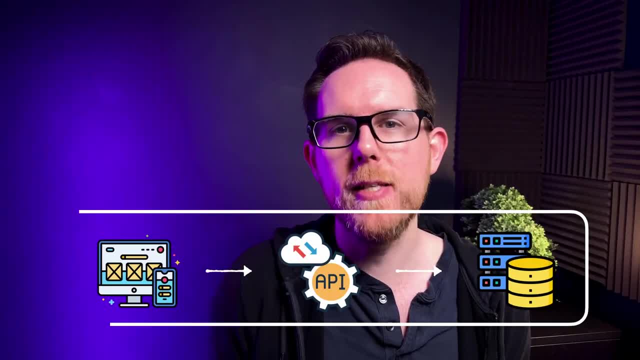 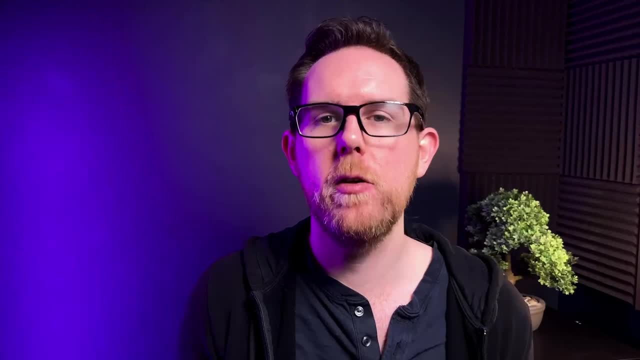 end-to-end tests need all the components working together and therefore they're typically run on an environment such as QA or UAT. It can take a while to have a stable set of end-to-end tests, especially if you're running them in a browser. Subtle things such as your application taking 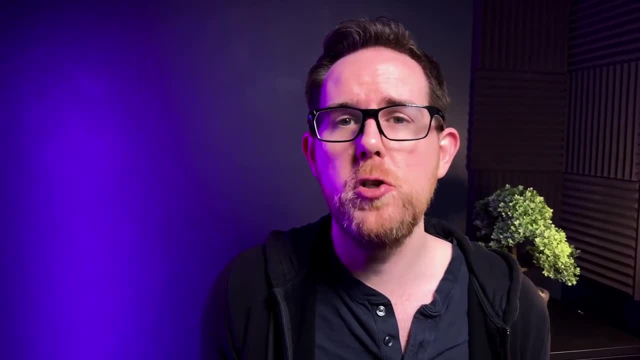 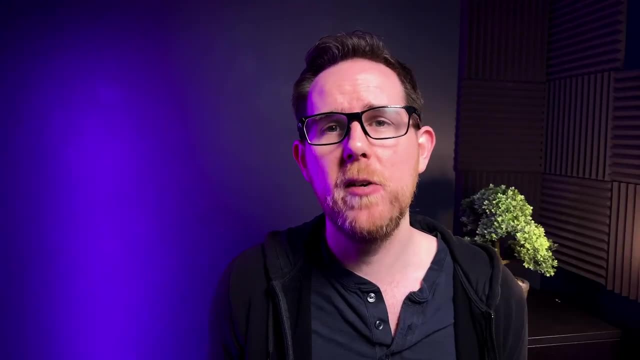 a little longer to load can cause your tests to break, and therefore you generally need someone working full-time on your automation tests. Many of the frameworks allow you to take screenshots when a test fails. This can be really useful to help you see what you're doing and how you're doing it. There are quite a lot of different tests that fall. 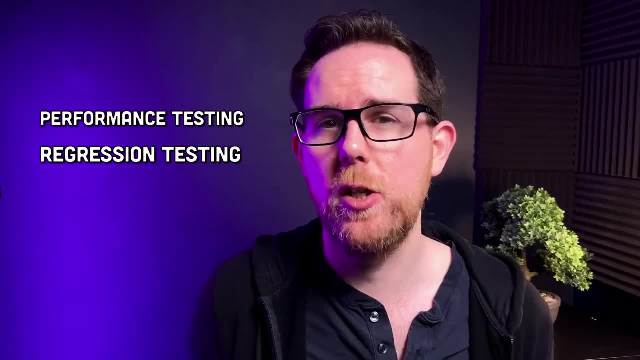 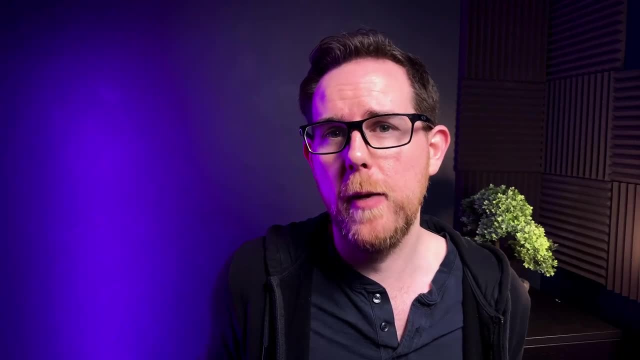 under this bracket, such as performance testing, regression testing and security testing. Finally, at the very top of our pyramid, we have the manual tests. These are the tests that are either too complicated to try and automate or they're not worth the time in trying to do it. Usually it's a 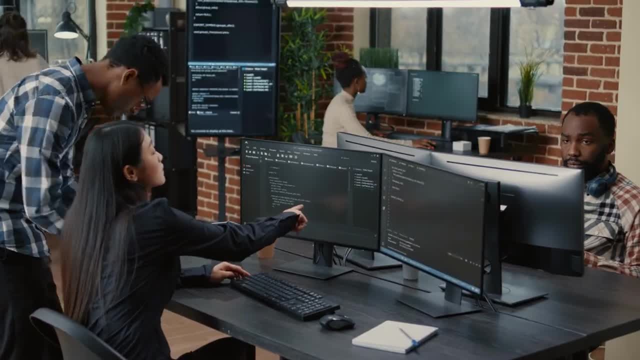 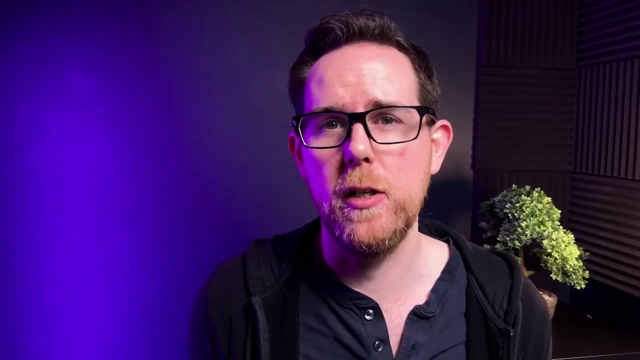 case of having not enough testers to developers, which results in tests having to be run manually instead of automating them. Ideally, you want to have the majority of your tests automated, otherwise you're going to be in this vicious cycle of not having enough time to test your application before. 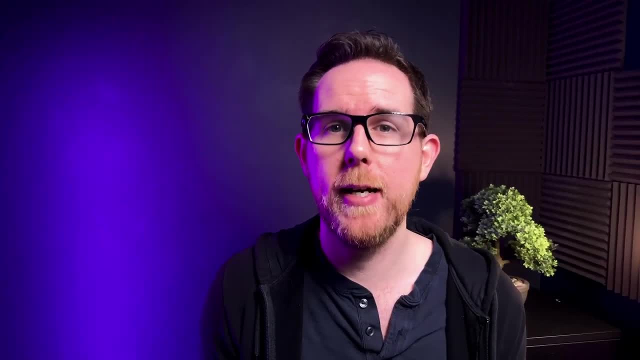 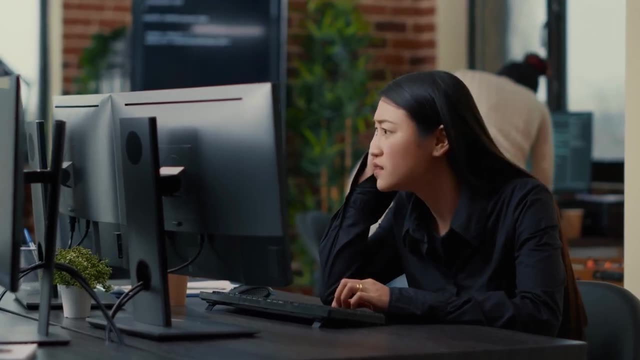 you can do it. If you find a bug in your application, then it's always better to find it lower down the pyramid than it is near the top. Let's say you find a bug while you're doing your manual testing. You now have to search for your logs and try and work out where exactly your